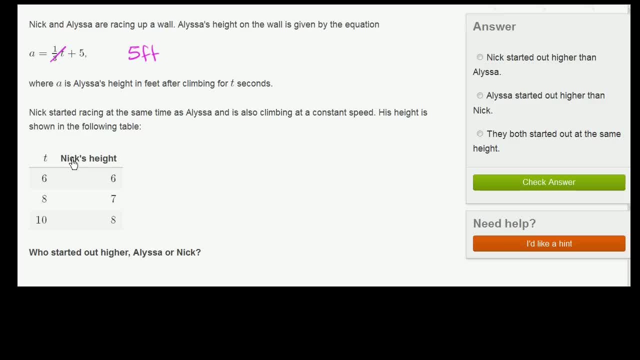 Now let's think about Nick's height at time equals 0.. And there's a couple of ways that we can go about doing this. One is just to back up, to kind of go backwards on this chart. So let me show you what I'm talking about. 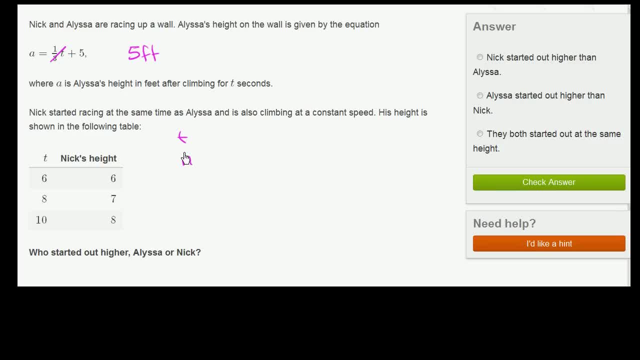 So, if this is time, and this is, let's say, n for Nick's height, because we have a for Alyssa's height. So let me make a little table here. We already know that at time 6 seconds or after 6 seconds. 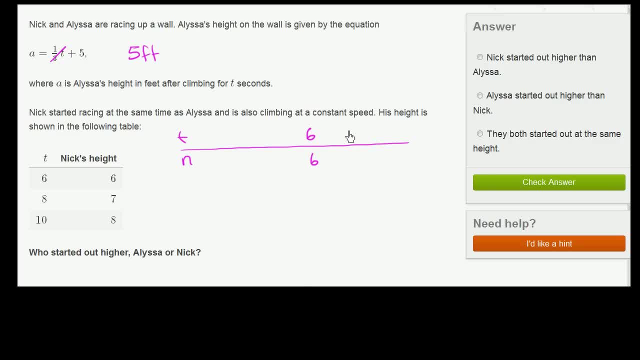 he's 6 feet in the air or along the wall. At time 8, he is 7 feet in the air or along the wall, And at time 10, he is going to be gotten to a height of 8 feet. 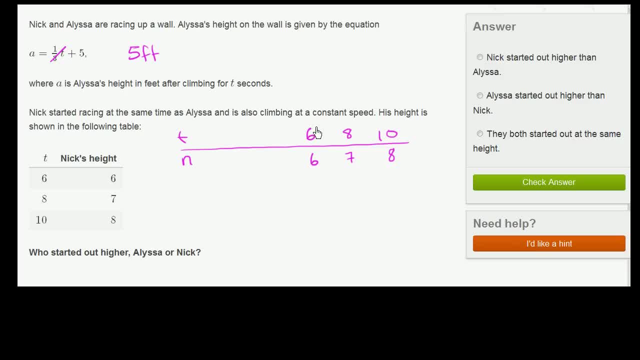 So what's happening here? Every time 2 seconds goes by, he increases in 1 foot. You have another 2 seconds, he increases in height by 1 foot. So you could go backwards If we take away 2 seconds to 4 seconds. 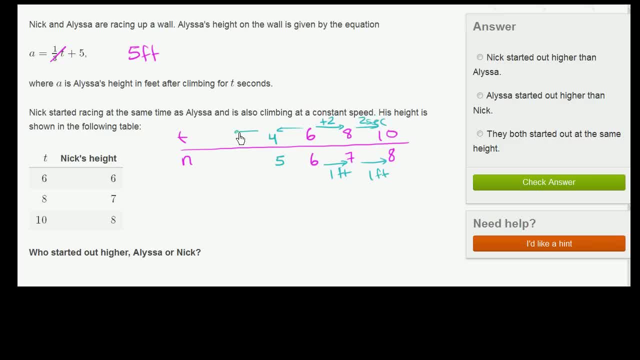 he will decrease in height by 1 foot. If we go back another 2 seconds, he will decrease in height by another 1 foot. The reason why we can say this is because we know he's climbing at a constant speed. So if we decrease by another 2 seconds to our starting time, 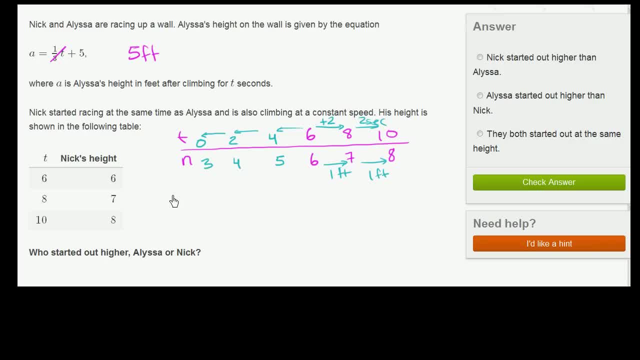 then we know that he would have been 1 foot lower, So he would have been at 3 feet. So just like that we now know time equals 0.. Nick's height is 3 feet in the air, So Alyssa started out higher than Nick. 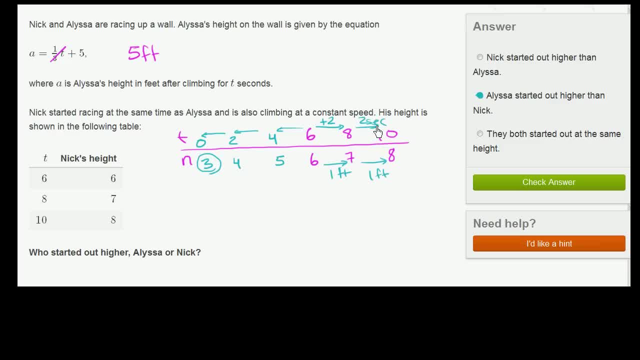 So this right over here would be the correct answer. Now the other way to do it is set up an equation, just like we had for Alyssa, and substitute for time equals 0. And the way to do that is to recognize that Nick's height as a function of time. 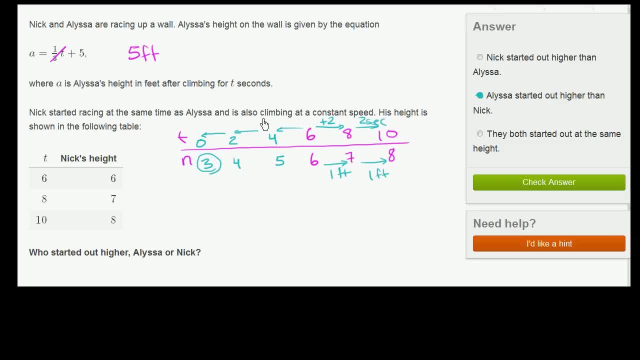 is also going to be a linear equation because they're both climbing at constant speeds, Or we know that Nick is climbing at a constant speed, So Nick's height, as a function of time, is going to look like. Nick's height is going to be some slope, some rate of change. 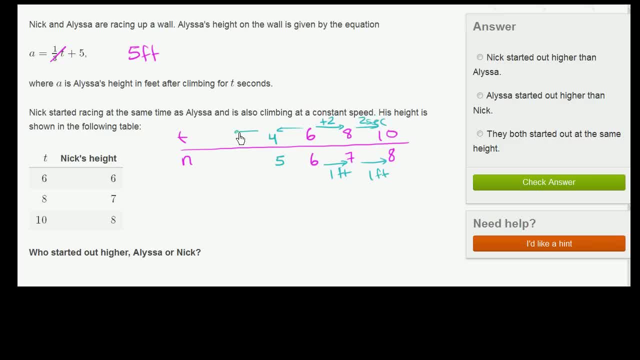 he will decrease in height by 1 foot. If we go back another 2 seconds, he will decrease in height by another 1 foot. The reason why we can say this is because we know he's climbing at a constant speed. So if we decrease by another 2 seconds to our starting time, 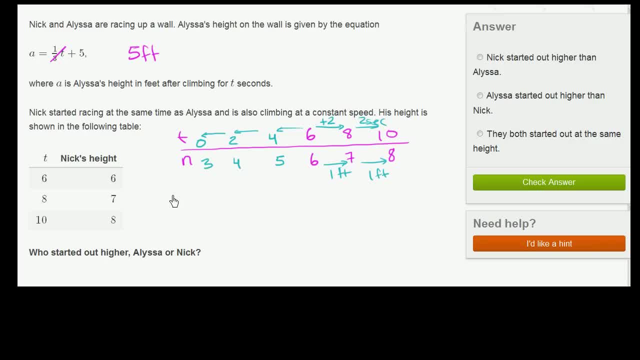 then we know that he would have been 1 foot lower, So he would have been at 3 feet. So just like that we now know time equals 0.. Nick's height is 3 feet in the air, So Alyssa started out higher than Nick. 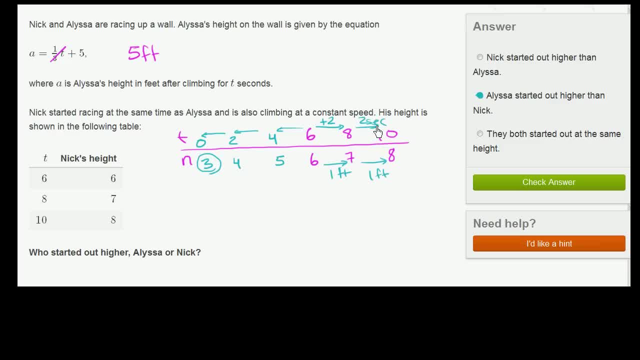 So this right over here would be the correct answer. Now the other way to do it is set up an equation, just like we had for Alyssa, and substitute for time equals 0. And the way to do that is to recognize that Nick's height as a function of time. 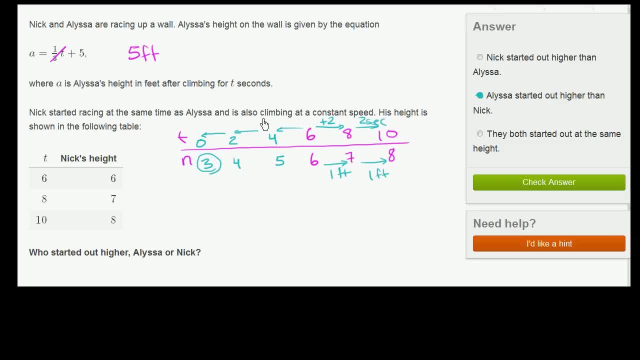 is also going to be a linear equation because they're both climbing at constant speeds, Or we know that Nick is climbing at a constant speed, So Nick's height, as a function of time, is going to look like. Nick's height is going to be some slope, some rate of change. 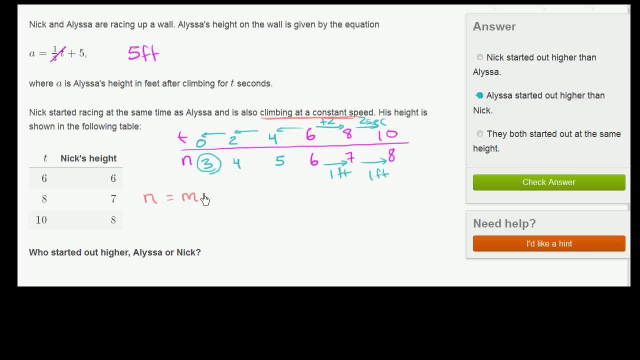 essentially his height per second times time plus his initial position. So how can we solve for m, the slope and his initial position? Well, the slope is just his rate of change of height, So it's literally how much does his height? 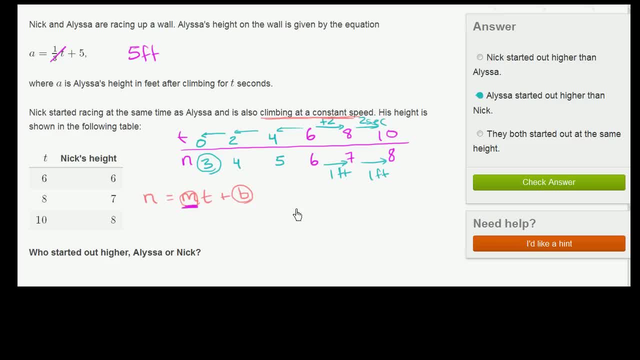 change per unit time. So m right over here, m is just going to be for a unit time, for a change in time. how much is his height changing? And his height is, we use the letter n. So we already know that when time increases by 2,. 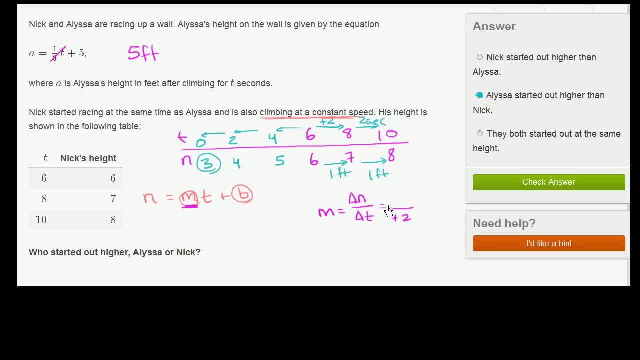 when time increases by 2, his height increases by 1 foot. So we know that m is equal to 1 half. He increases 1 half feet per second And you see that there, because it takes him 2 seconds to go 1 foot. 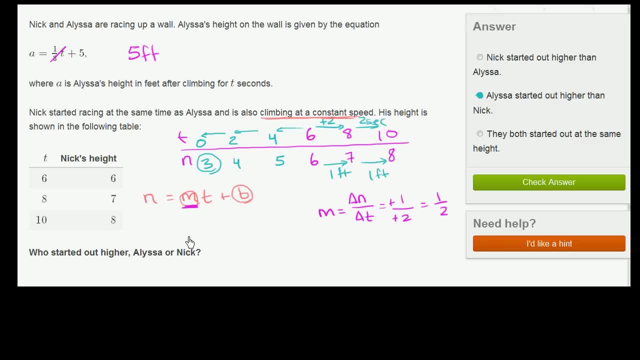 So we can fill in m here. So we know now that n is equal to 1 half t plus b. Now to solve for b, you could just substitute one of these points. All of these points must satisfy this equation right over here. 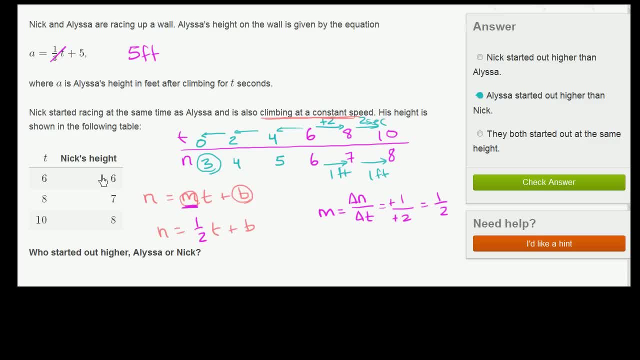 So we could use the point 6.. So if we put a 6 in here, so when time is 6, we know that n is 6.. So you have: 6 is equal to 1 half times 6 plus b. 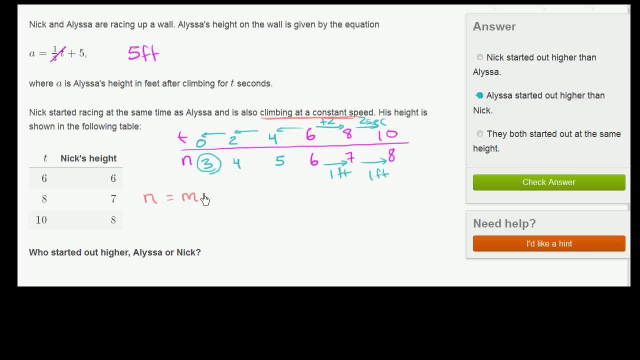 essentially his height per second times time plus his initial position. So how can we solve for m, the slope and his initial position? Well, the slope is just his rate of change of height, So it's literally how much does his height? 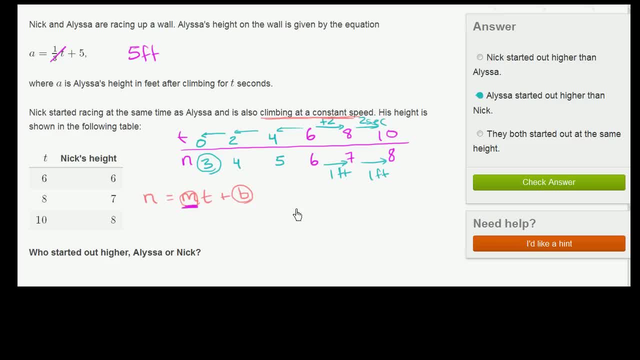 change per unit time. So m right over here, m is just going to be for a unit time, for a change in time. how much is his height changing? And his height is, we use the letter n. So we already know that when time increases by 2,.